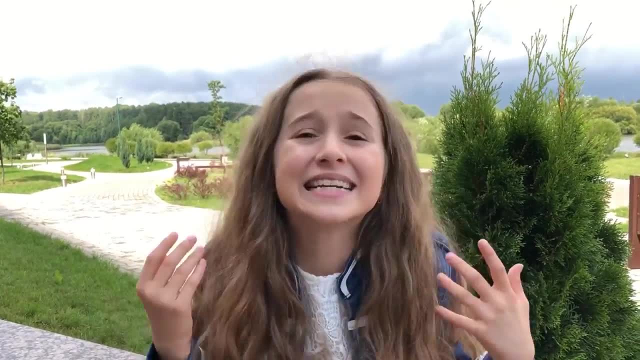 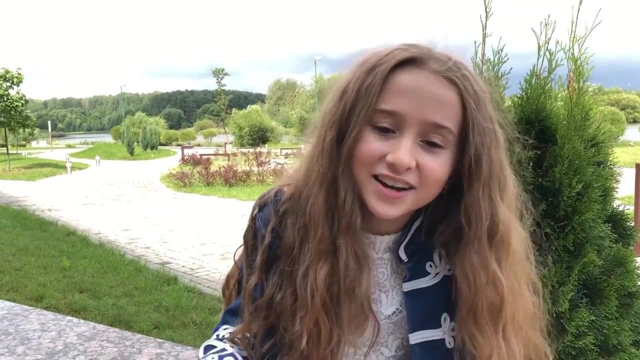 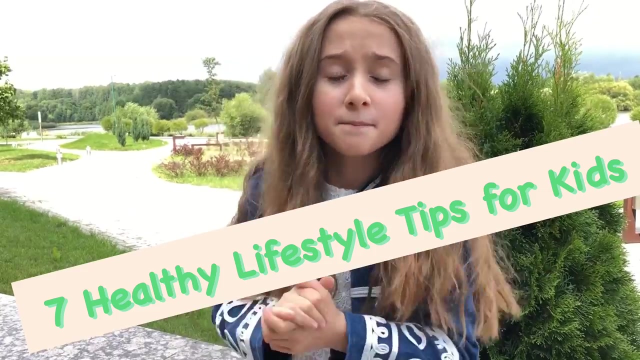 Hello YouTube. how are you? At last, the school year is over and it finally feels like summer- Yay: No responsibilities, no homework, no pressure and loads of free time. So I thought it would be a perfect time to introduce you to some healthy changes to your life. 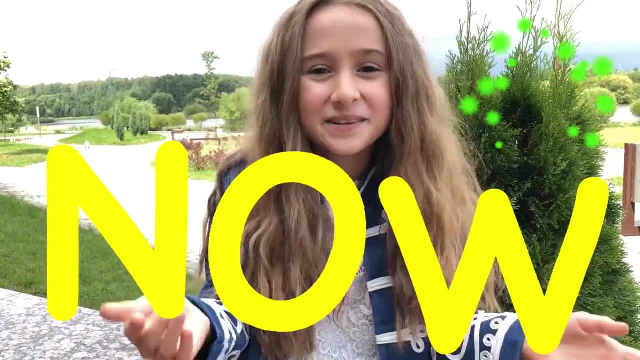 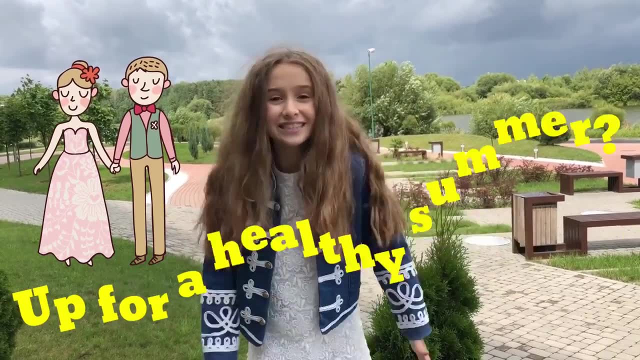 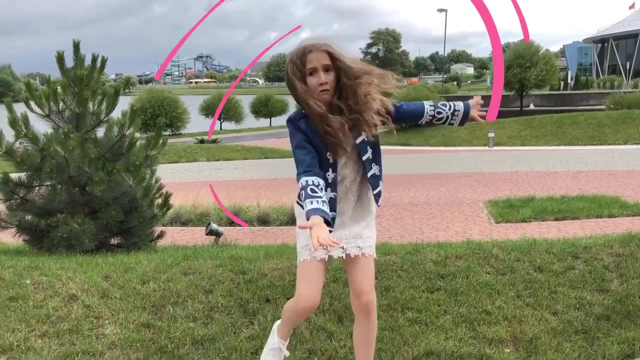 If you want to change your life, the best time is now. So I thought: why not grab your family and friends to go on a healthy challenge together? Do you think that's a good idea? The first step is always the hardest. You don't have to be great to start, you have to start to be great. 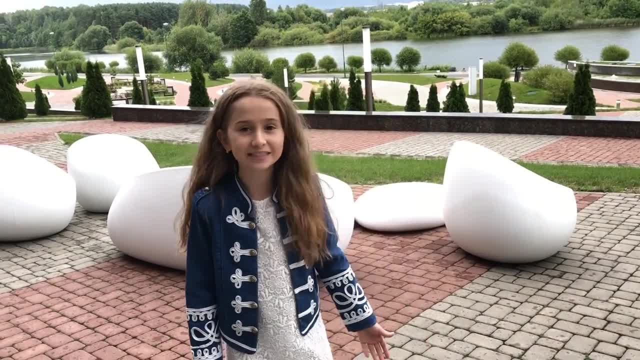 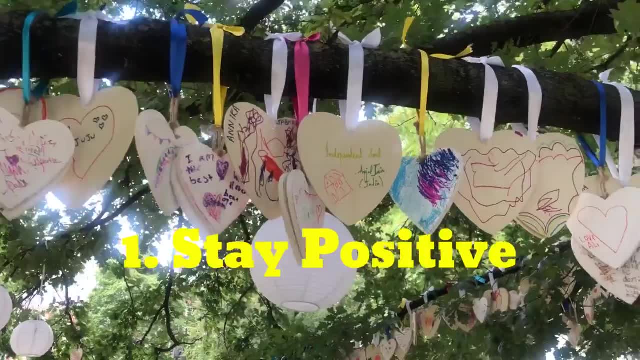 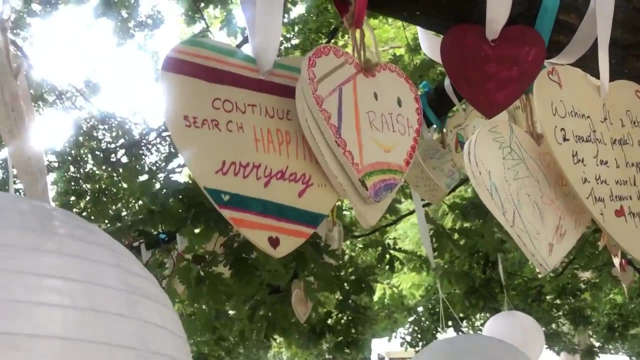 So I thought I'd give you a few healthy tips to get us all started. Please comment to add a healthy tip of your own. Number one: stay positive. Positive attitude helps us build a happy life and happy attitude helps us be healthier. When life gives you lemons, make lemonade. 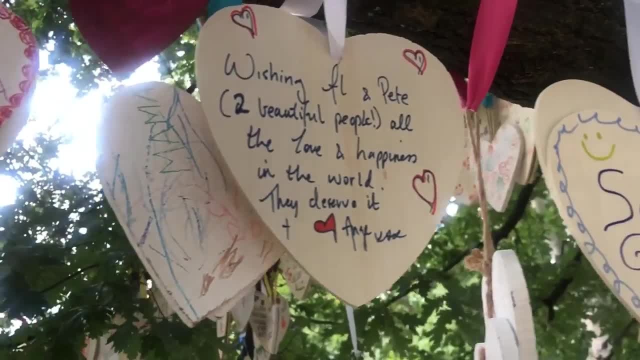 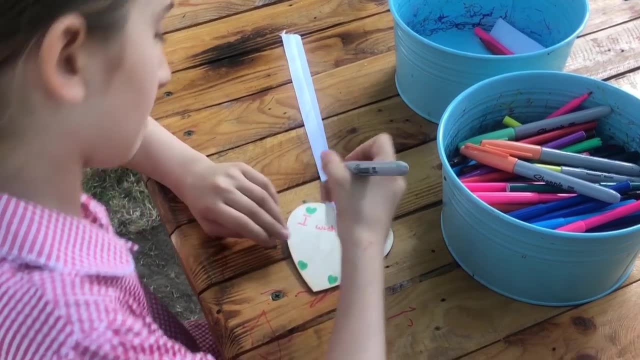 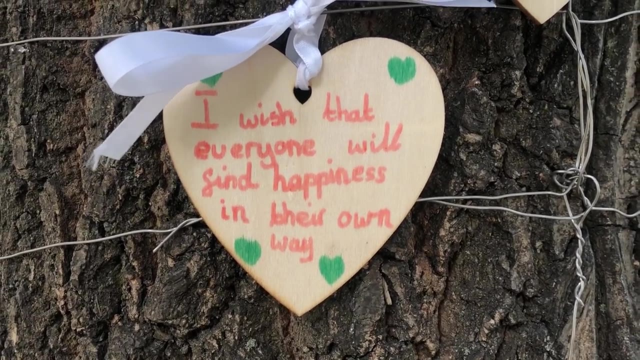 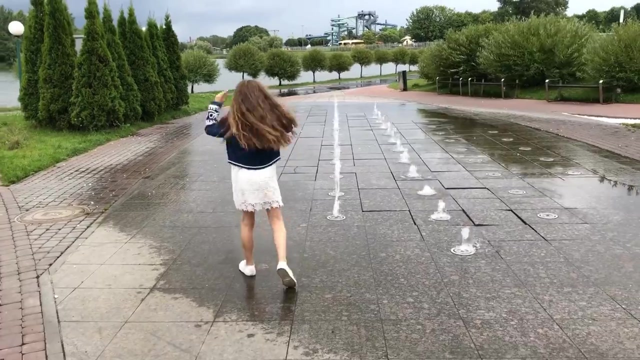 We can start with telling each other that we are beautiful and amazing, and encouraging each other to learn new things and celebrate each other's successes. Number two: drink plenty of water. Do you know that up to 60% of the human body is water? 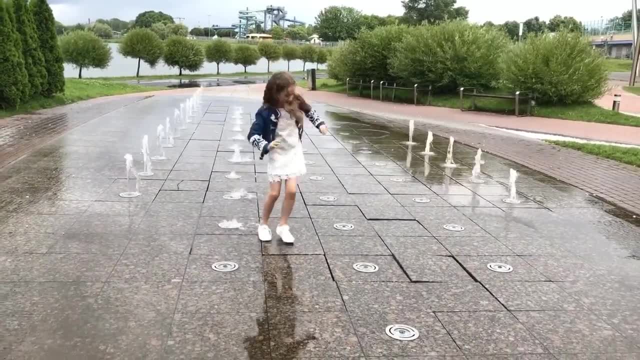 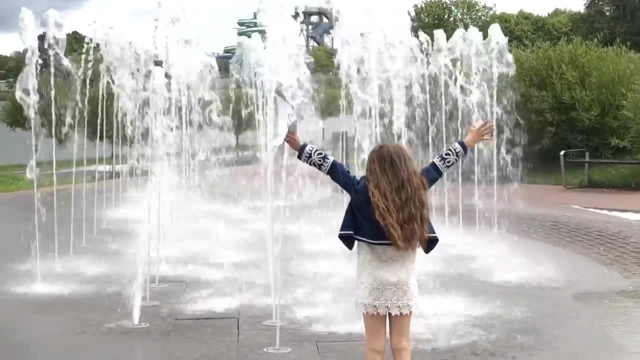 Our brains and hearts are composed of 75% of water and the lungs are about to 83% water. The skin contains 64% water and even the bones are watery- 31%. So water is super important. Thank you, Thank you. 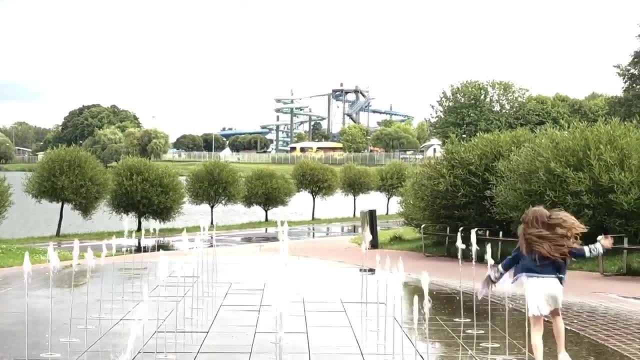 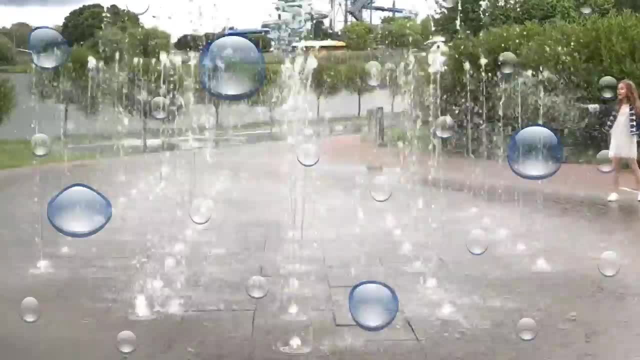 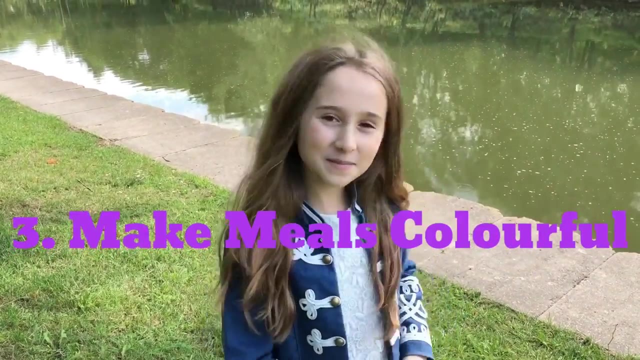 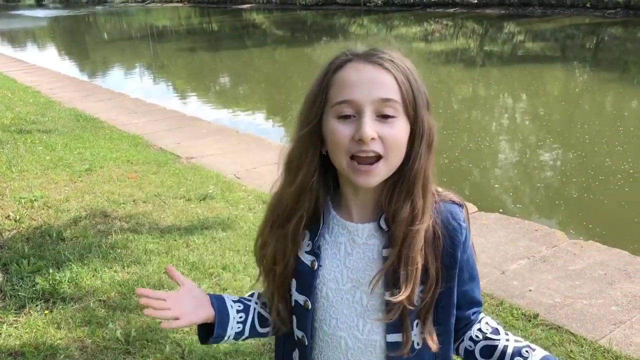 It helps us build energy, takes food to our organs and helps us survive. Tip number three: make meals colourful. Eating is about staying healthy. One idea is to add as many brightly coloured foods as possible to each plate you eat. Red for apples, green for apples. 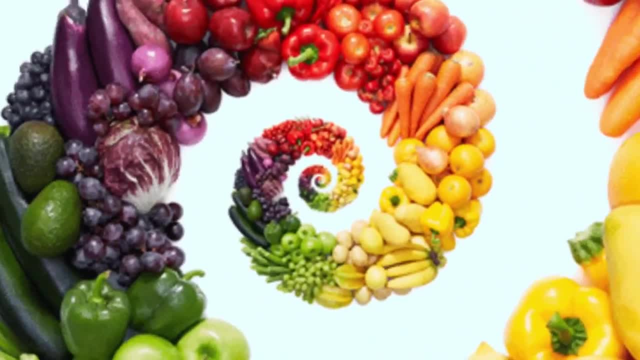 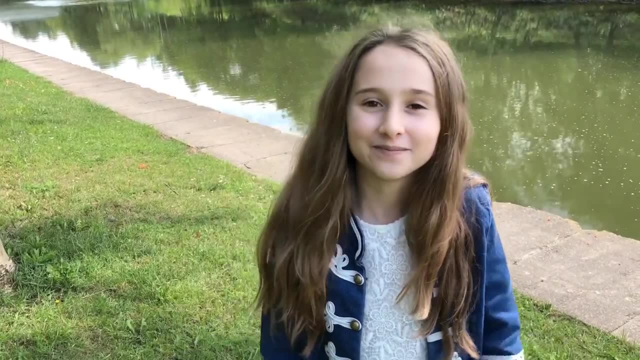 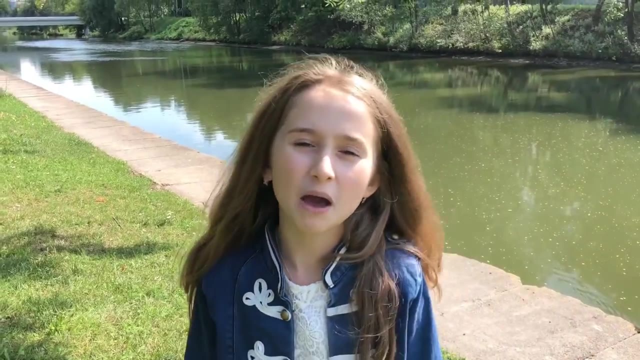 For avocado, broccoli beans, Orange is for oranges and carrots, Pink for watermelon And, lastly, white for cauliflower. Tip number four: get enough sleep. In one of my recent videos, I spoke about how important it is to get enough sleep.